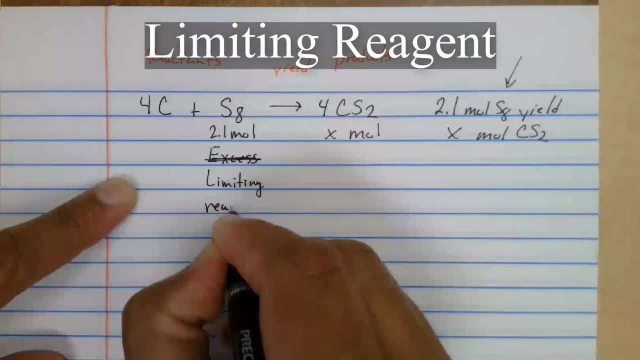 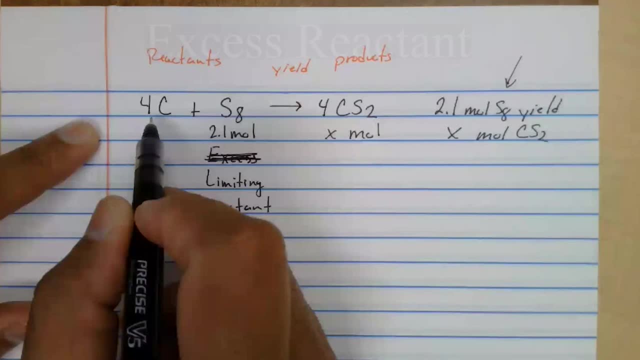 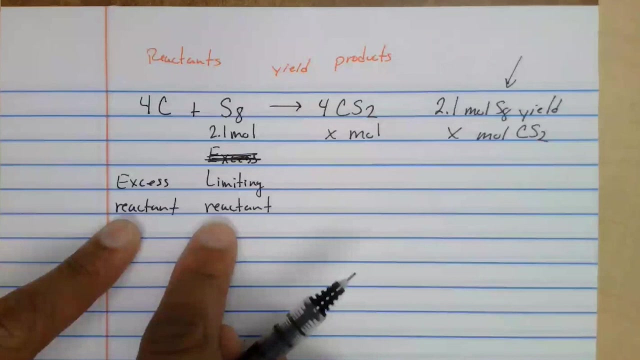 In some books you'll see limiting reagent. It's the same thing. They don't tell us anything about the carbon. so, right there, we just assume that this is the excess reactant. The reaction is limited to this: 2.1 moles of sulfur. 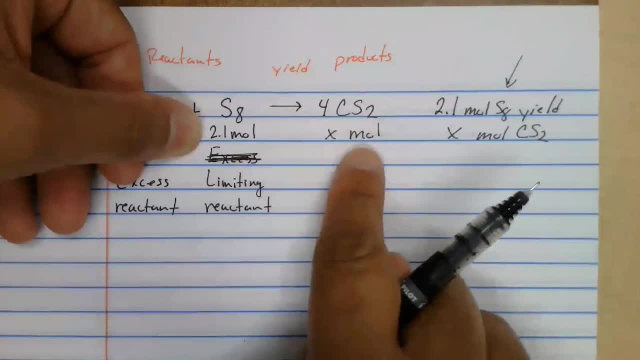 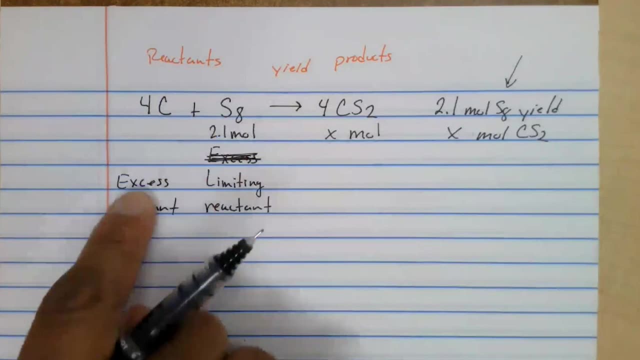 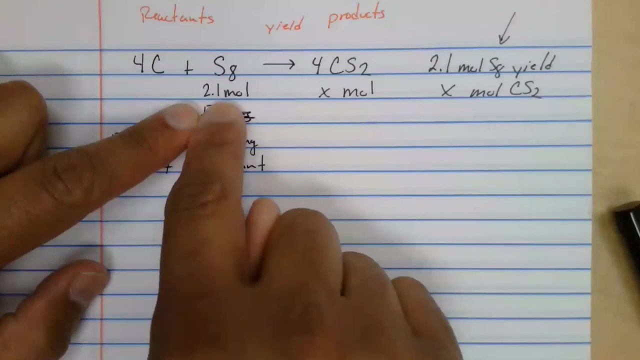 So the amount of product we get It's just dependent on this number. right here There's going to be carbon left over. Carbon will react, but this is not what's going to limit the amount of product. We want to convert the moles here to the moles here. 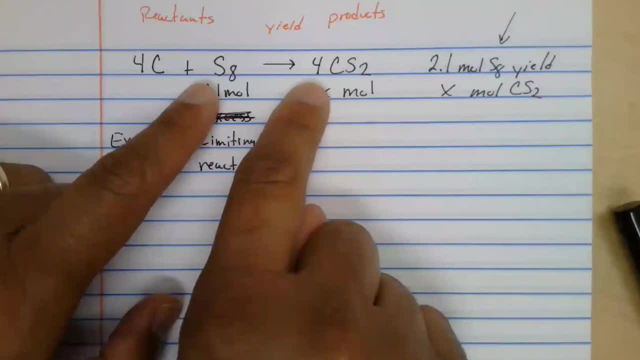 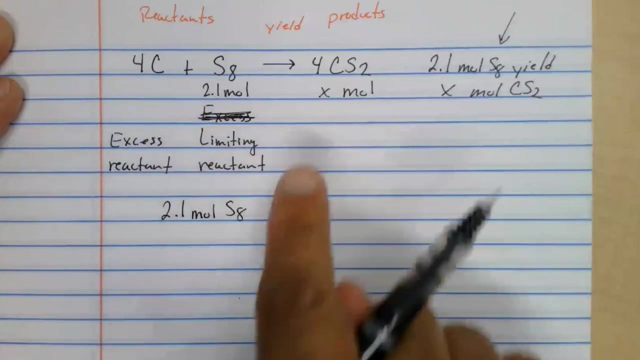 And we do that by knowing these. the mole ratio, the mole ratio of carbon disulfide to sulfur is just four to one. So watch how easy this is. 2.1 moles, Mole Of S8.. We want to convert. 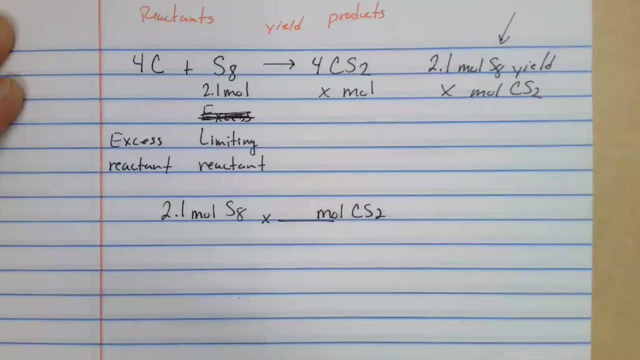 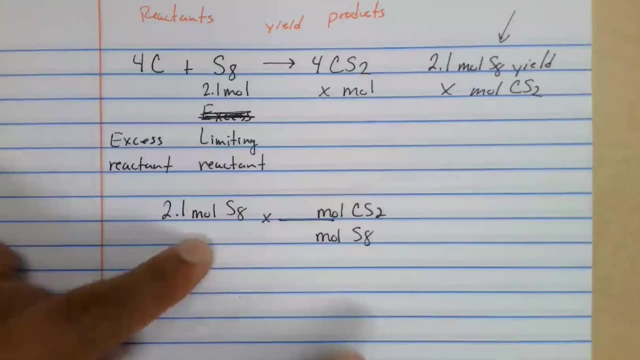 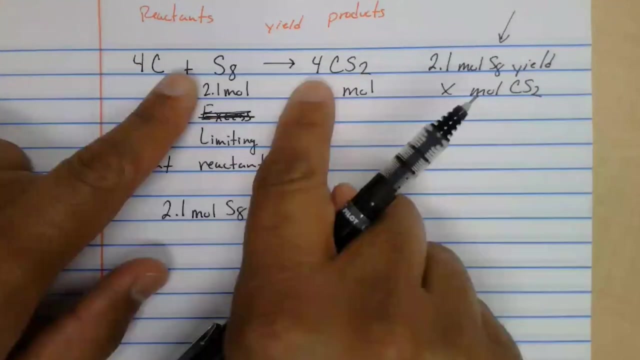 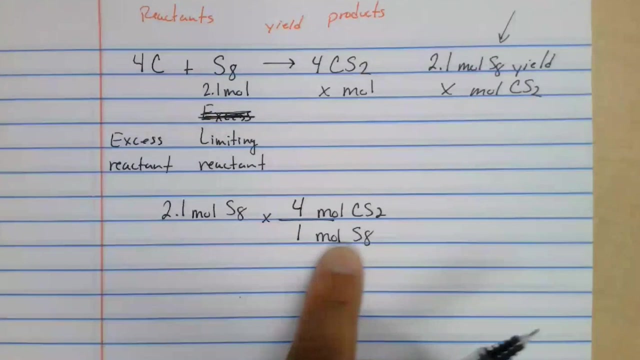 To the mole Of CS2.. Let's cancel the mole Of S8.. So when you see this mole to mole ratio right here Of carbon disulfide and sulfur, that comes right from our mole to mole ratio, For every one mole of sulfur that reacts you will always produce exactly four moles of CS2.. 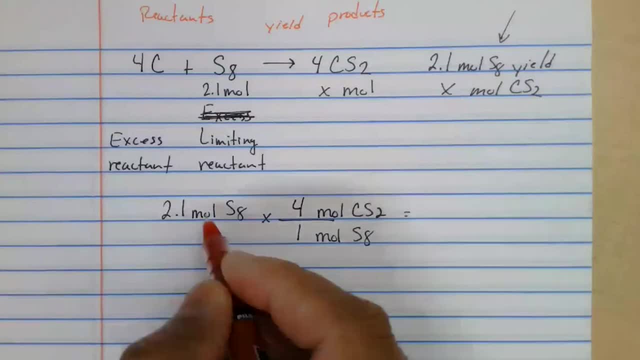 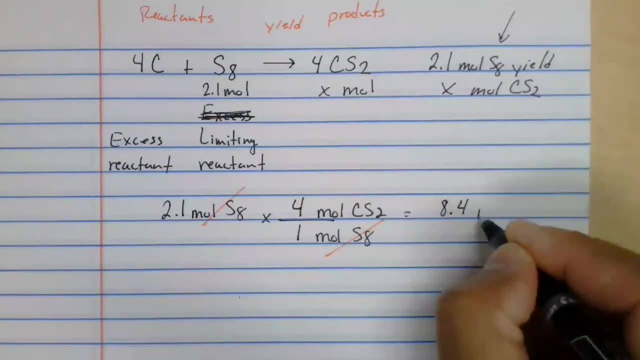 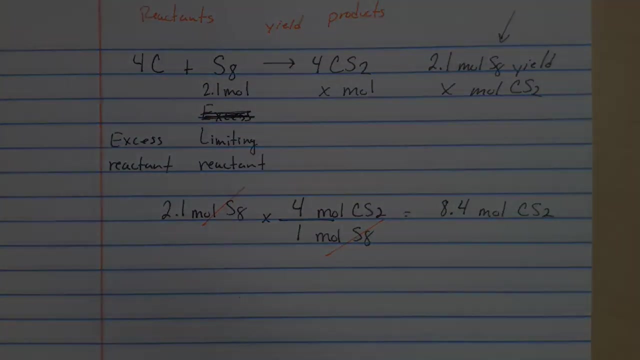 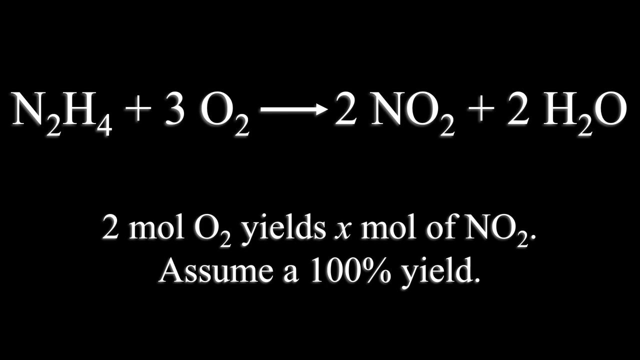 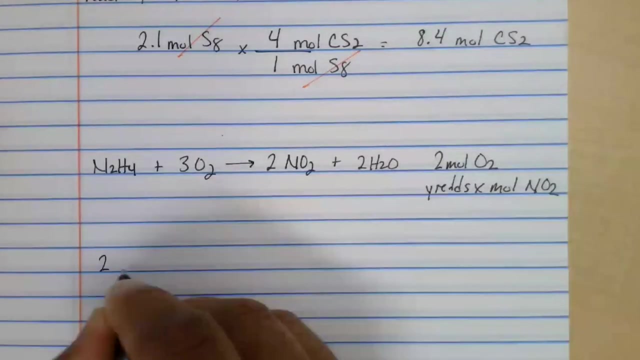 And that's it. If you understand this step right here, Then you can do any stoichiometry problem. So let me pause there, I'm just going to wait. have two moles of 02.. And we want to know from the two moles of 02.. 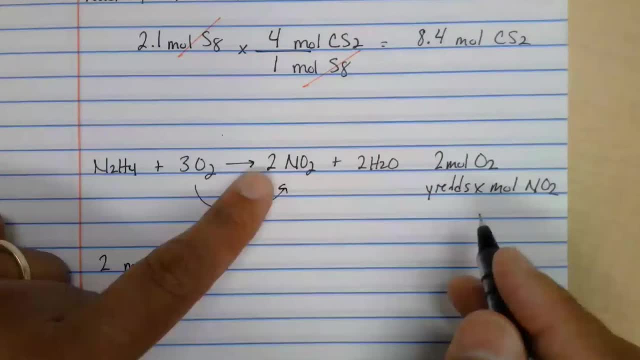 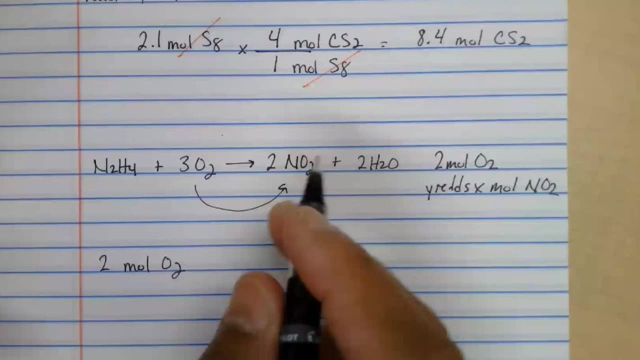 How much NO2. Of S8. is being produced, How many moles of NO2?? So just from this question, as we saw a second ago, I can just assume that this is our limiting reactant, because that's all I'm worried about. 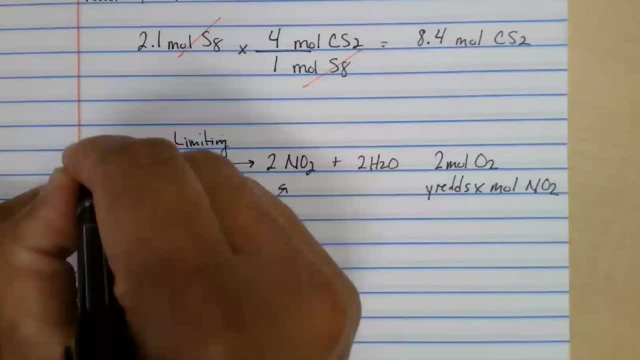 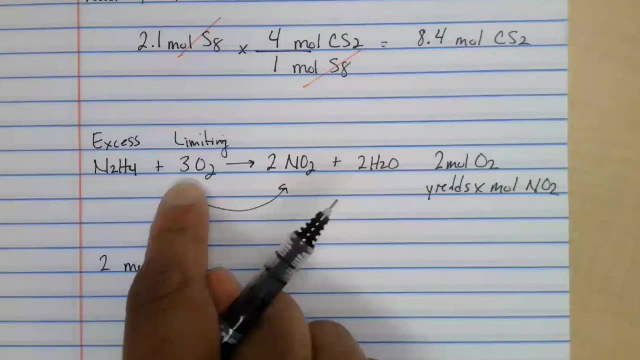 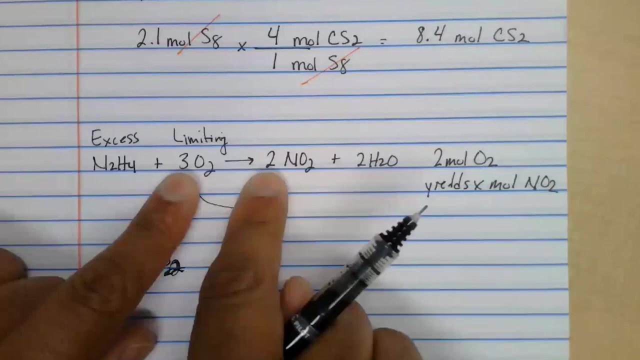 The hydrazine, this will be considered the excess. So the hydrazine will react with O2, but we just assume that this is excess, because all I'm worried about are these two moles of the O2.. Okay, so let's do it From unit of moles. we use the mole-to-mole ratio. 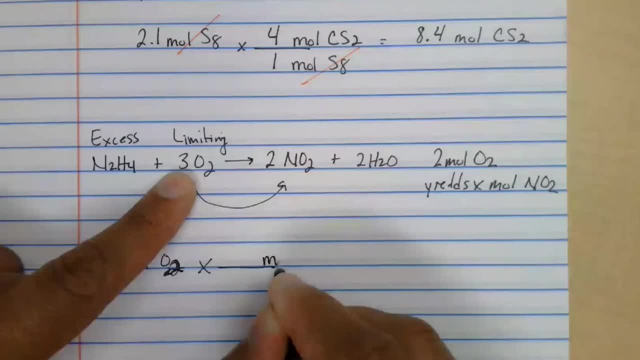 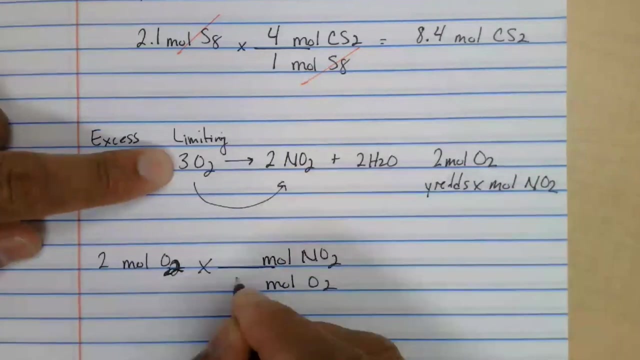 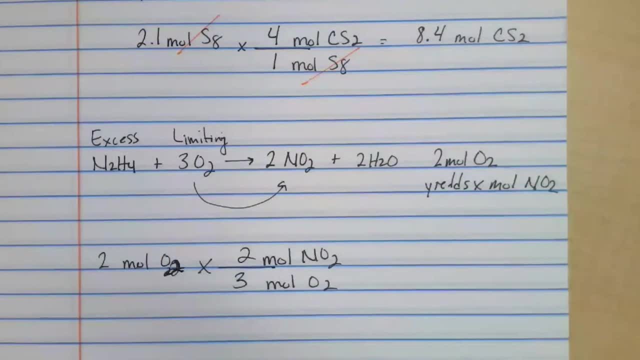 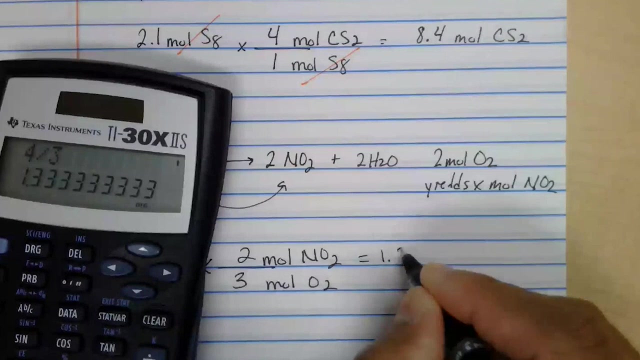 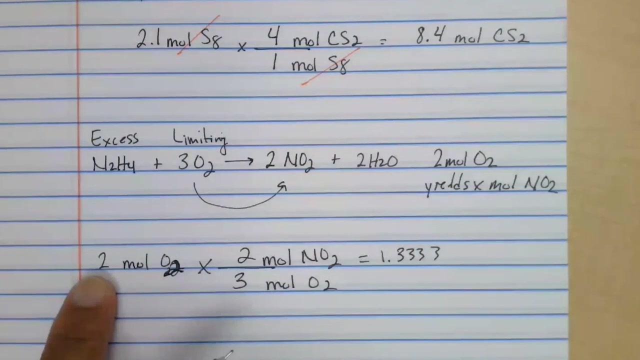 Two moles. Our answer should be one significant figure. So let's check that. Two times two is four. Four thirds is going to be 1.3333, whatever, But the answer should be one sig fig. So this is interesting. At least two moles. 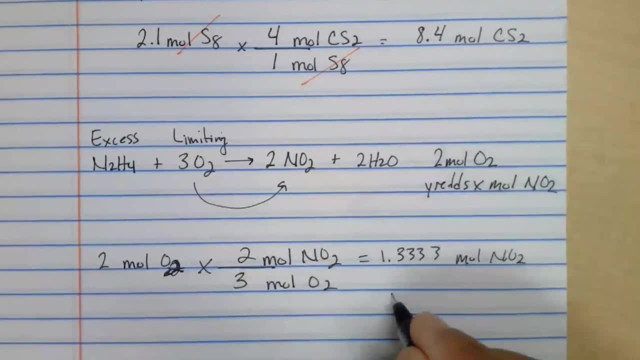 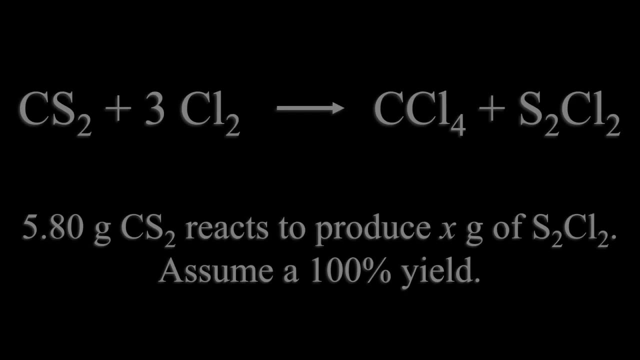 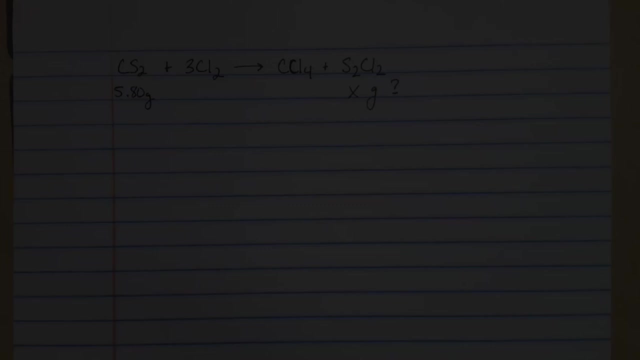 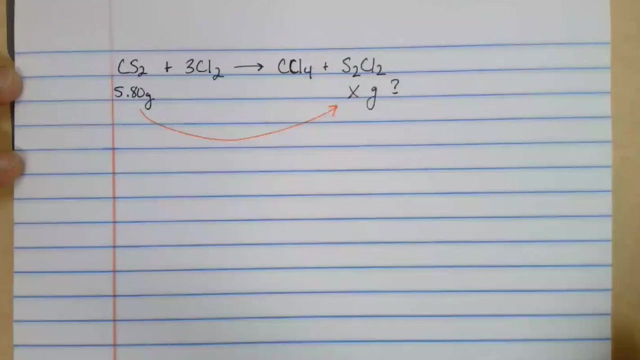 one significant figure that we're certain of this will be one mole of NO2.. We're doing the exact same problem: We want to find the amount of product, but instead of moles they give us the grams, and we want to find the grams. 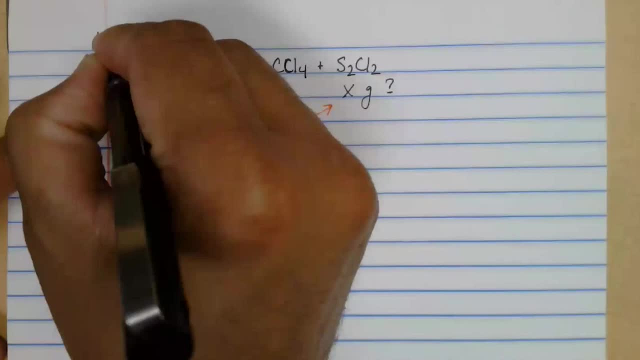 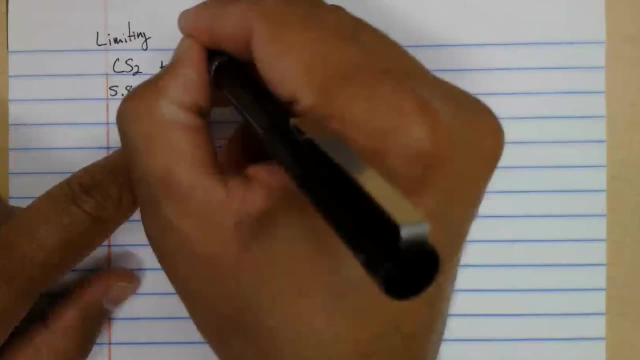 A couple things here. Number one: they tell us the limiting reactant, The one that they don't give us. the other reactant, of course, will be excess, so we don't have to worry about finding the excess. so we just assume that it's this one, because 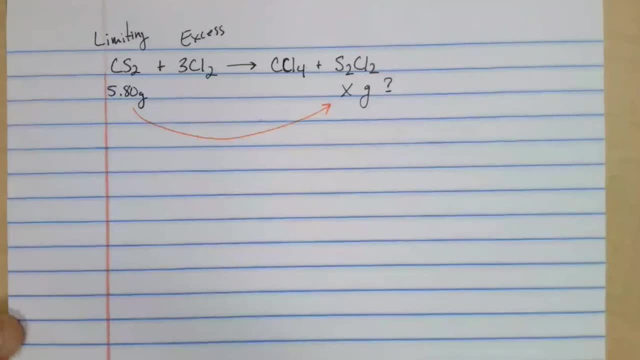 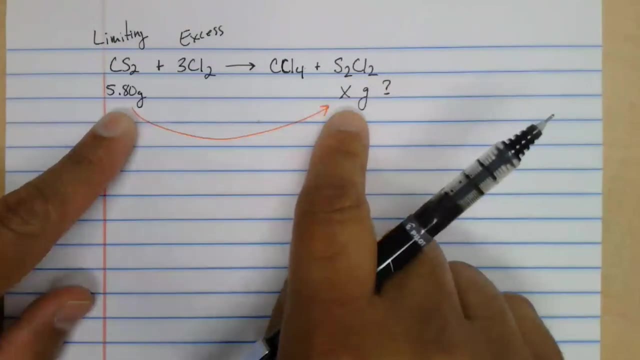 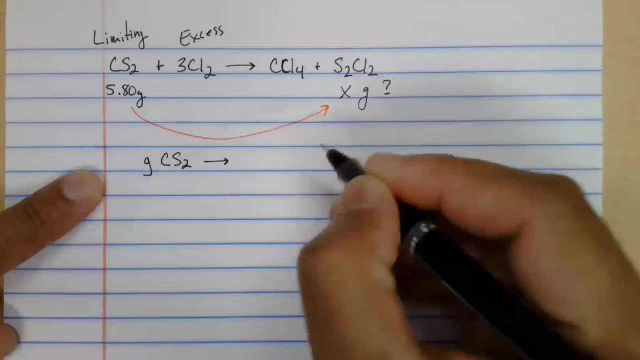 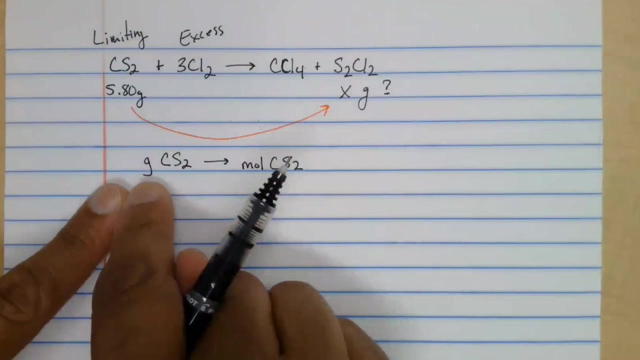 they don't tell us anything about chlorine. The rules of stoichiometry don't change. In order to find this relationship, we need units of moles. We're going to go from our grams- Grams of CS2, let's convert to the mole of CS2, and how do we convert grams to moles? 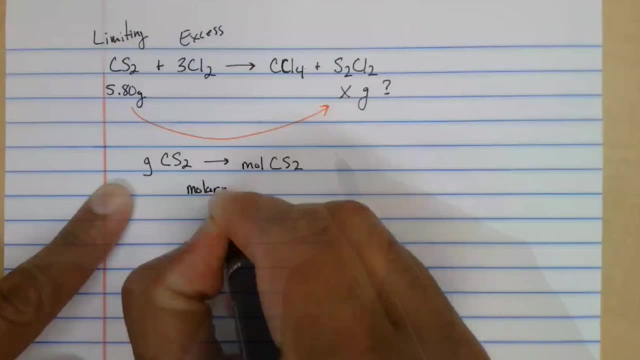 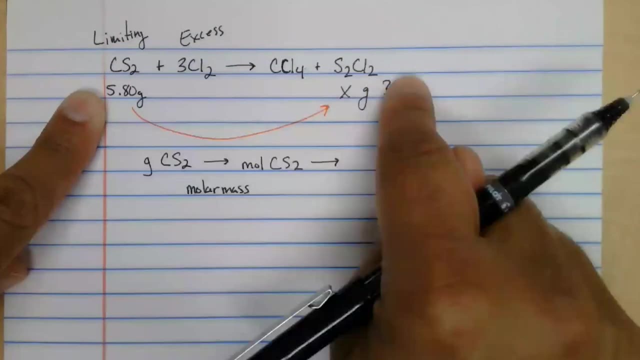 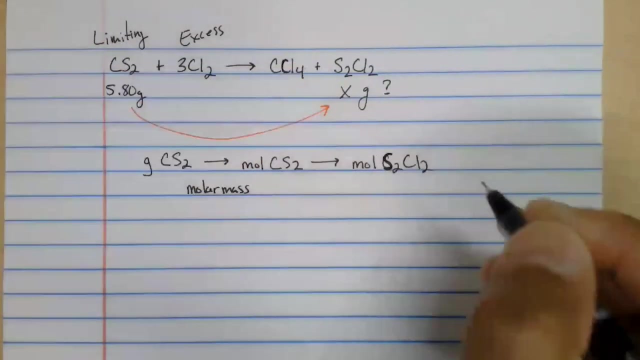 It's called the molar mass. Then we can convert to moles of anything whatever I want to look for. In this case we're going to go to mole of the disulfur Dichloride. They're asking for the answer in grams, so of course we can convert moles to grams. 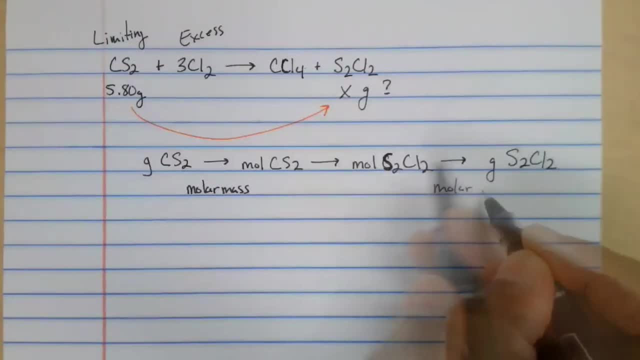 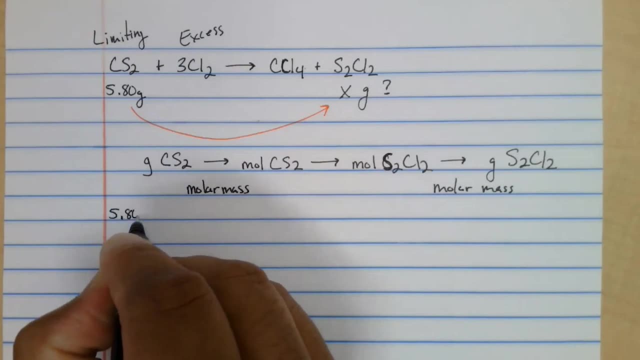 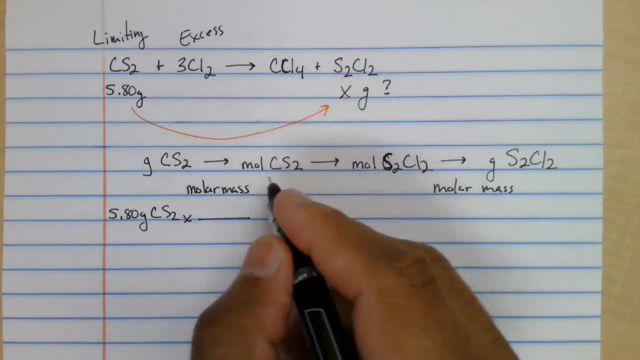 of disulfur dichloride and use the molar mass to convert the moles to grams: 5.80 gram CS2, multiply by a ratio. We want to convert to mole of CS2. And cancel the gram of CS2.. 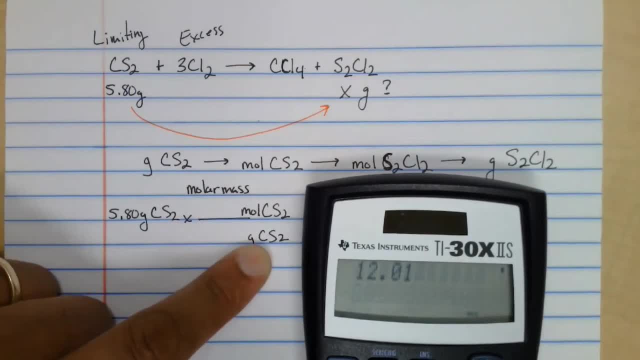 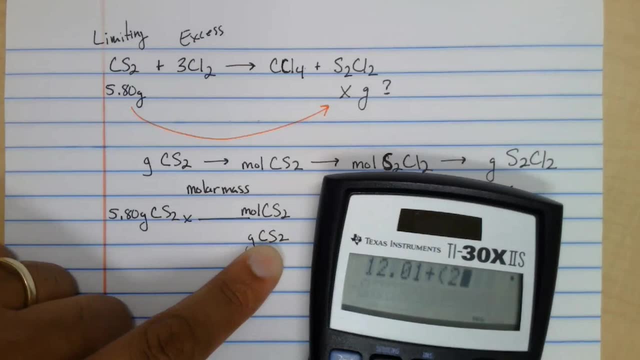 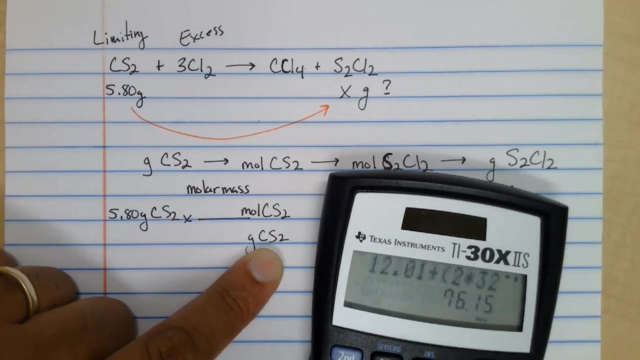 The molar mass. remember it's one carbon. so molar mass for one carbon plus two times the sulfur. Now sulfur on my table is 32.07.. So to two decimal places, that's good enough for our calculations. 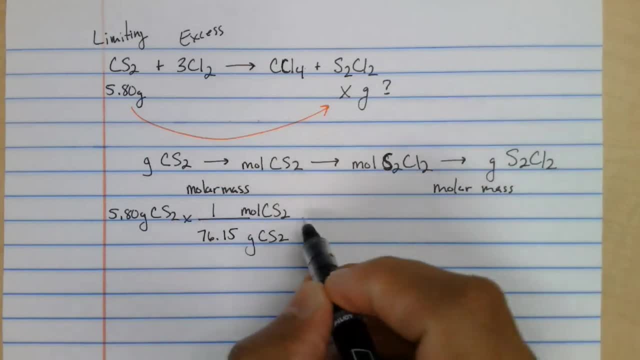 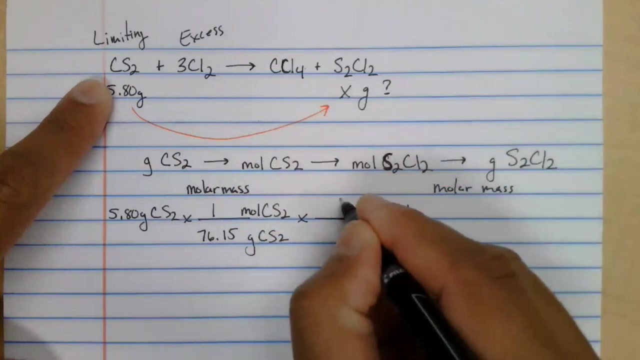 76.. 0.15 for the molar mass, The mole-to-mole ratio. again we're looking at our balanced equation. Now this is pretty convenient. This is just one-to-one. For every one mole of CS2 that reacts, you will always produce one mole. 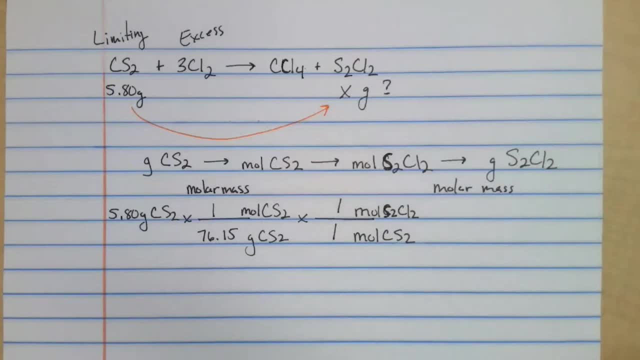 For every one mole of CS2 that reacts, you will always produce one mole Of the S2Cl2.. Right here at the end, we've already solved the answer. but they're not asking for moles of product. They're asking for the grams of product. 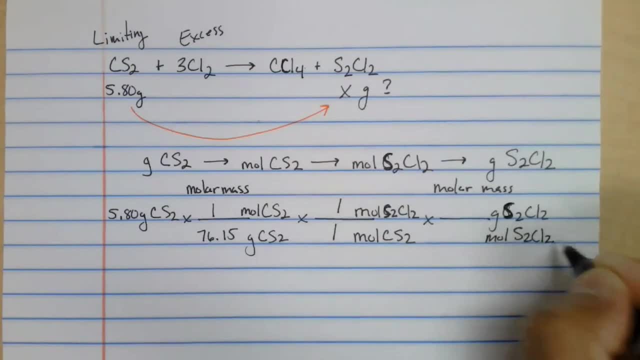 So right here, S2Cl2.. Here we have the molar mass for two chlorines plus two sulfurs. Okay, So the mole mass is 16.5 times the total 43.2.. So we're going to run a comparison and say if we're interested in seeing how much. 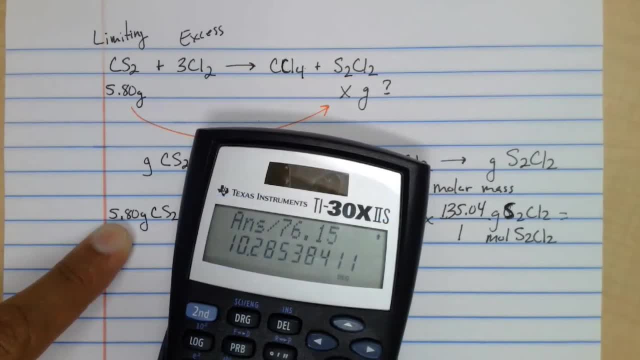 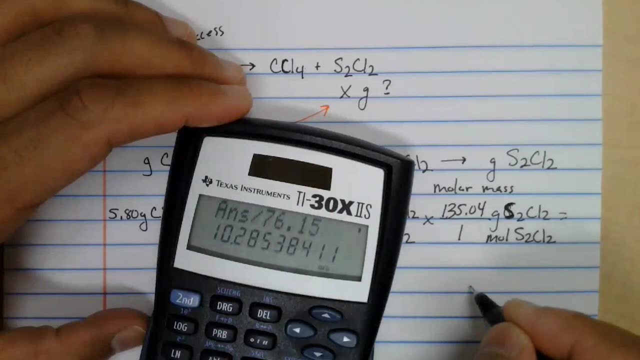 molar mass we can produce. if we're not sure if that's the ideal number, let's check that out, And in the next slide I'm going to show you a comparison with different hogs. So right here we start with three sig figs. 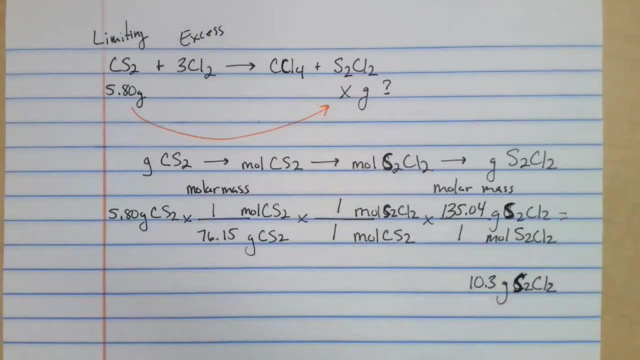 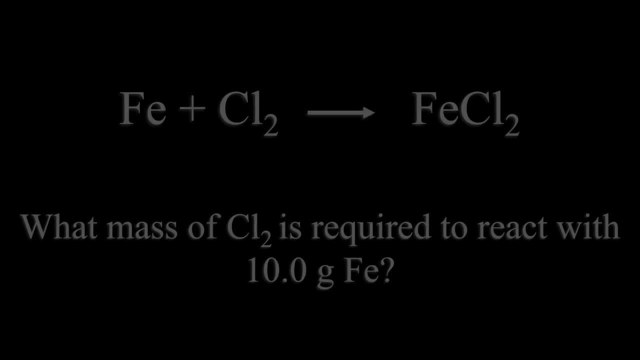 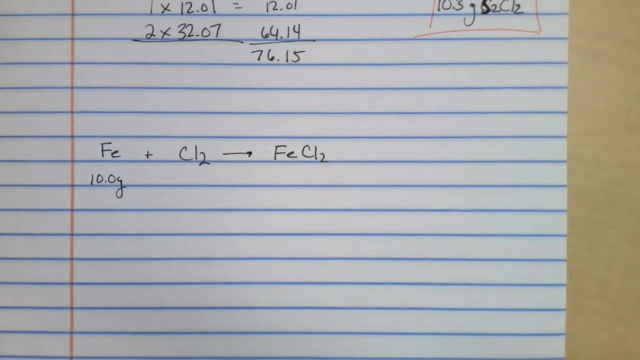 So our answer should have three sig figs, So I'll answer 10.3.. Okay, Okay, Okay, We're going to get out of here. Let's get going a little bit different in the last examples that we've done. we've done three examples so far and 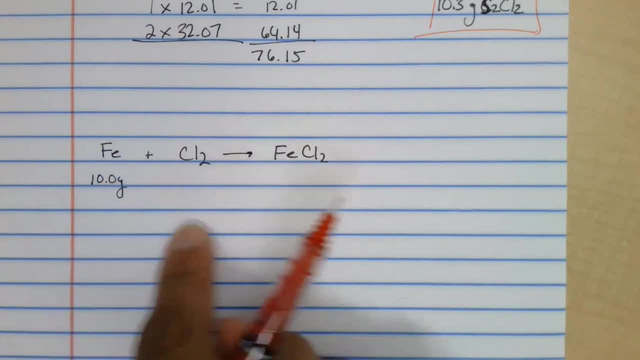 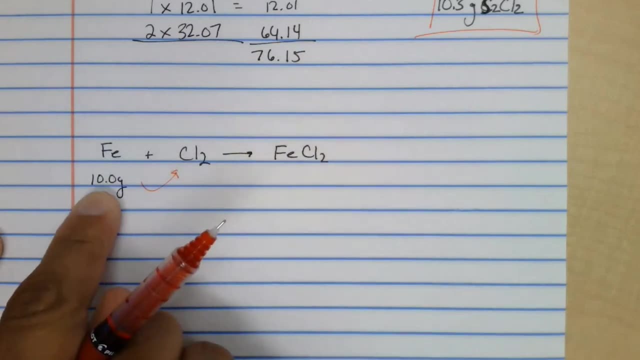 in each example we converted a reactant to a product. but this question is interesting because it's asking: well, if i start with this amount, how much chlorine do i need to completely react? and, by the way, for your engineers, some of you going into chemical or petroleum engineering- 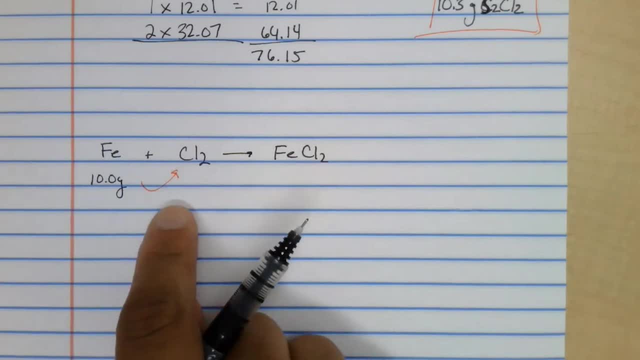 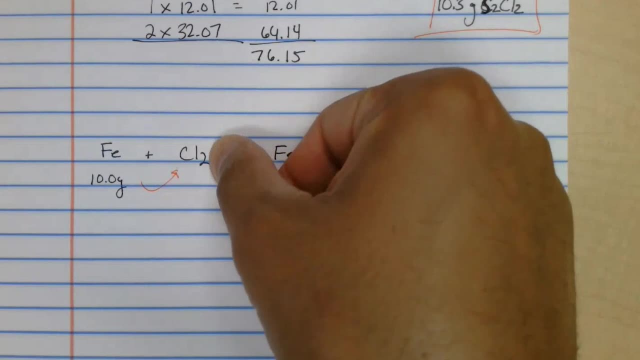 this is really a really important stoichiometry problem. so you want to minimize the amount of reactant you use. you don't want anything extra. you don't want to spend your money and buy more than what you really need. you want to spend just the right amount. 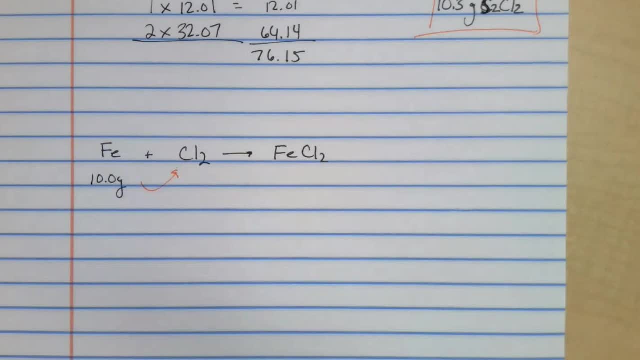 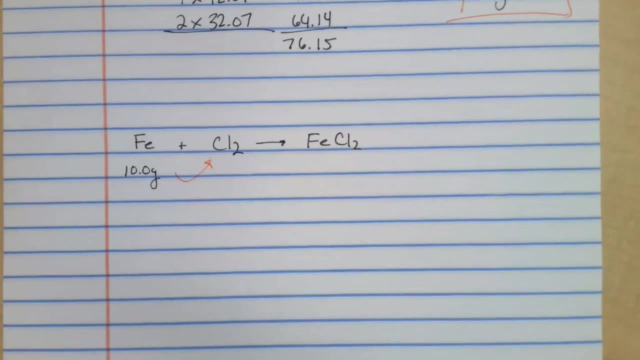 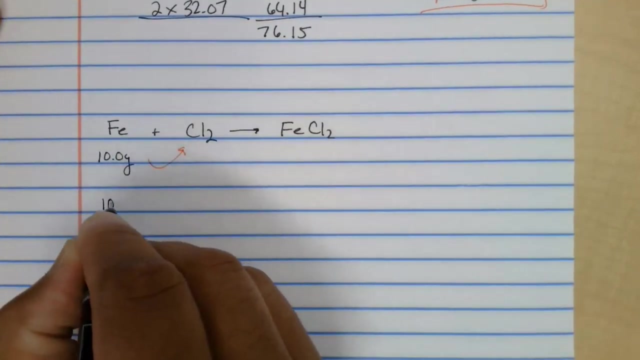 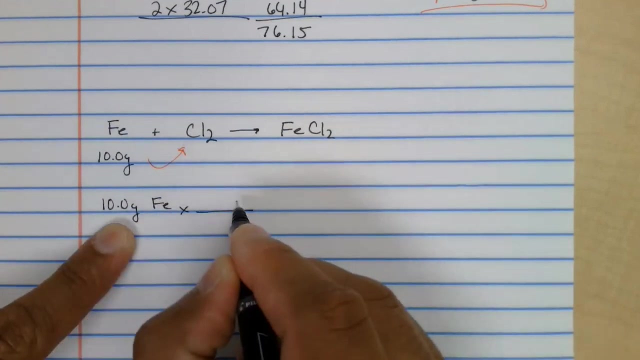 on exactly what you need. so that's part of the cost efficiency for you know, those of you that are going to come across that and everyone, every one of you- will come across cost efficiency at some point. so this is actually a very important problem: to find the moles of iron. 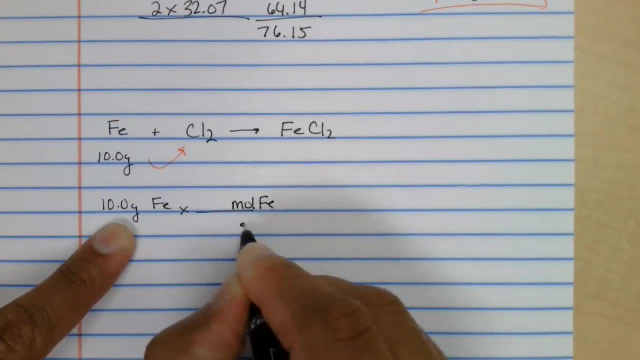 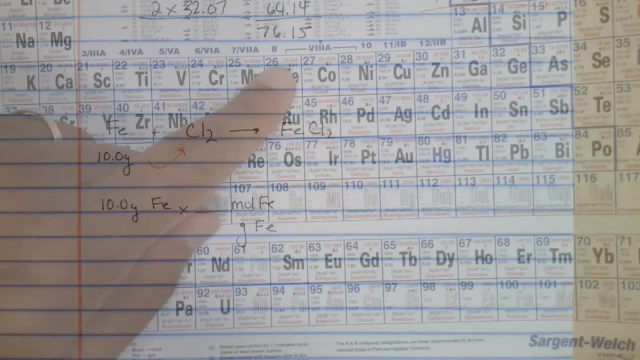 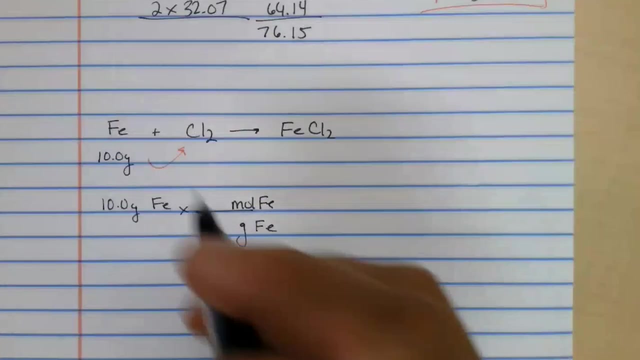 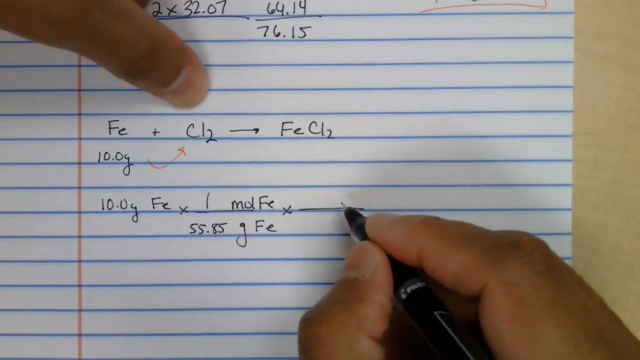 we divide by the grams of iron, and that comes from the periodic table, this is a 55.845, but we'll round to two decimal places. that's good enough for our calculations. now that we have moles of iron, now we can convert to whatever we want. in this case we're converting to a reactant mole of chlorine and cancel the mole. 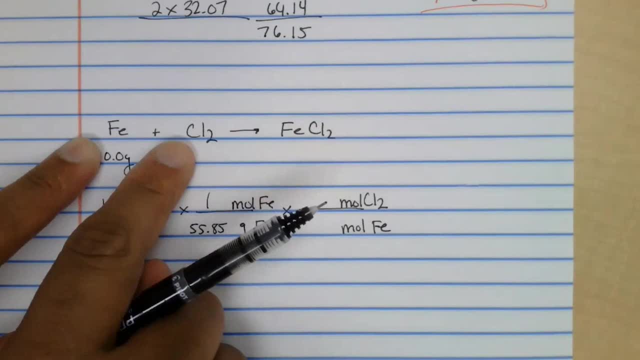 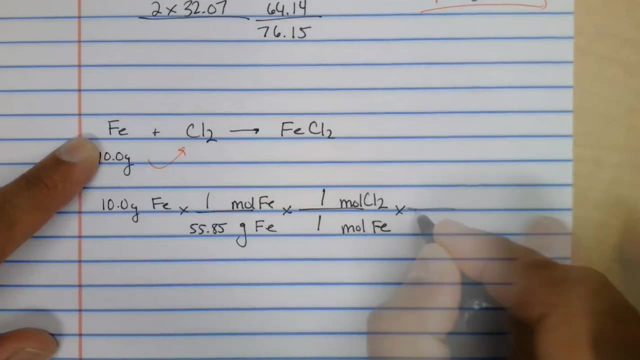 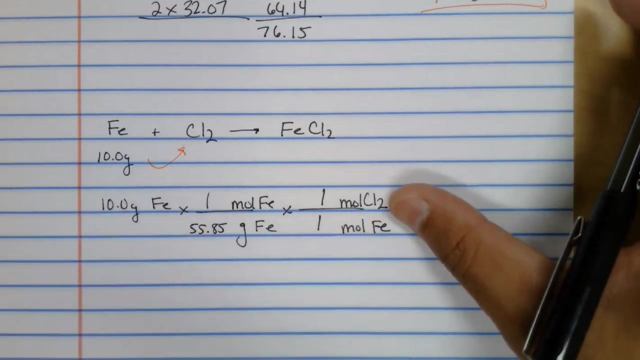 of lactate iron right here pretty convenient. this is a simple one-to-one ratio. so again, that comes from the balanced equation. we already did it. we found the amount of chlorine in terms of moles. but be careful: sometimes we ask for moles, sometimes we ask for grams. so in this case they're asking for. 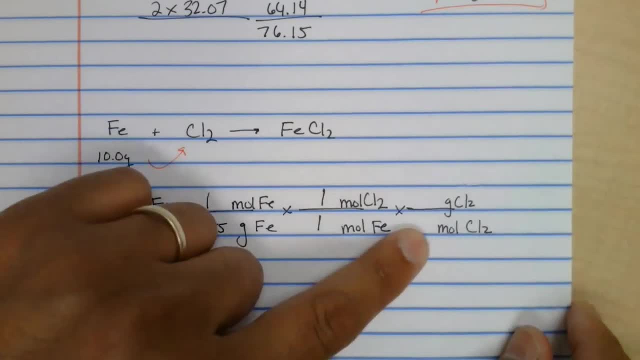 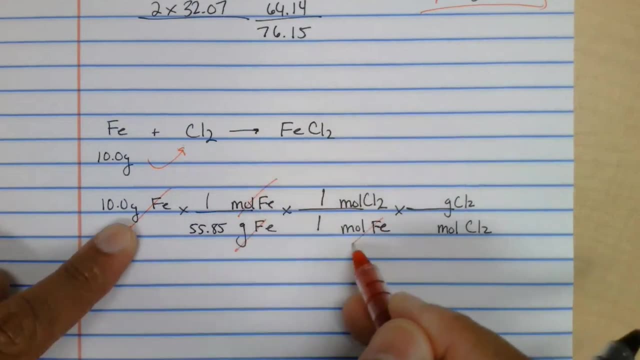 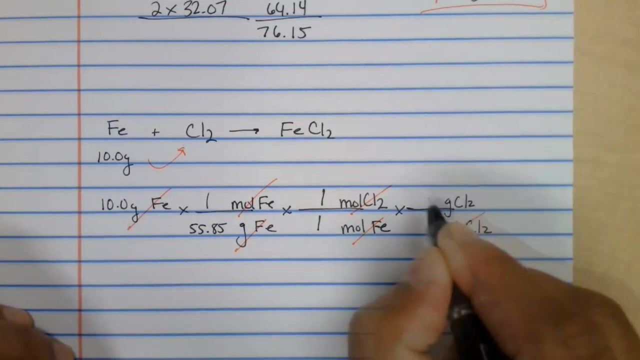 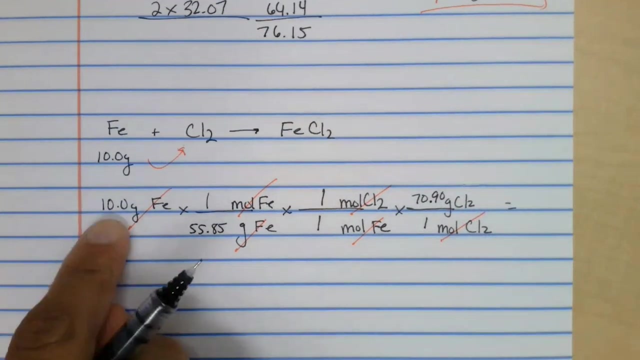 the grams of cl2. i use the molar mass to cancel these units out. check those units, see how all these units cancel it. all makes sense here. so the final answer is in grams. chlorine is two chlorines, so 70.90. i start with three sig figs. my answer will have three sig figs, 12.. 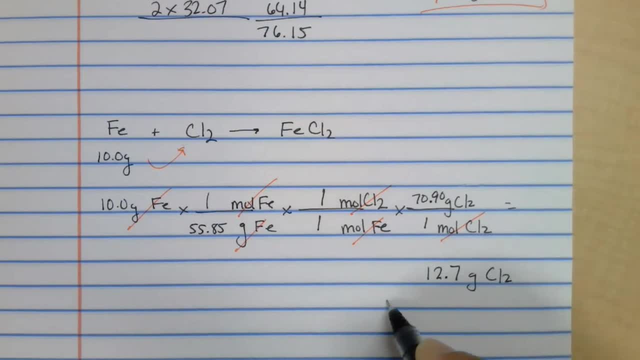 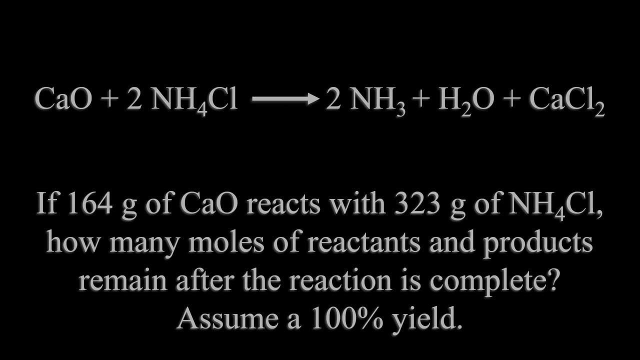 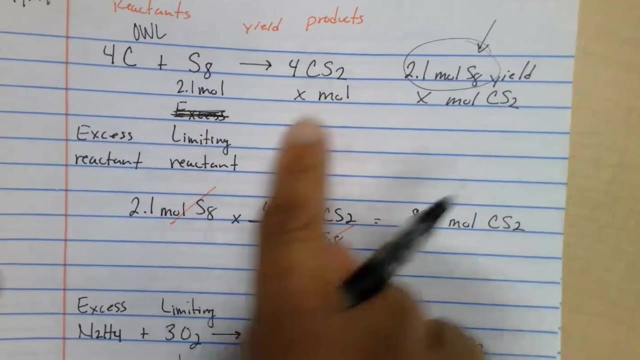 seven grams of cl2 will completely react with 10 grams of iron. that's the significance here. that's what this number means. this number represents the amount of chlorine that reacts with all of the iron. in our previous questions they told us: well, this is how much reactant we have. 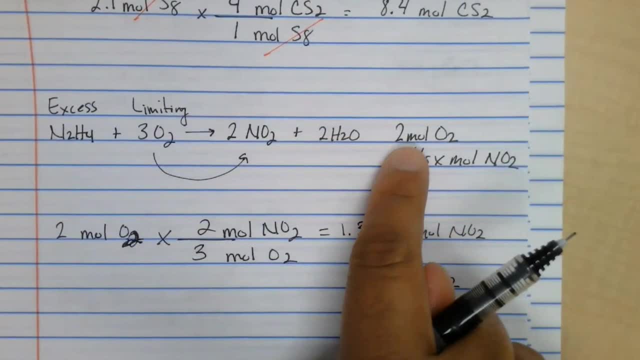 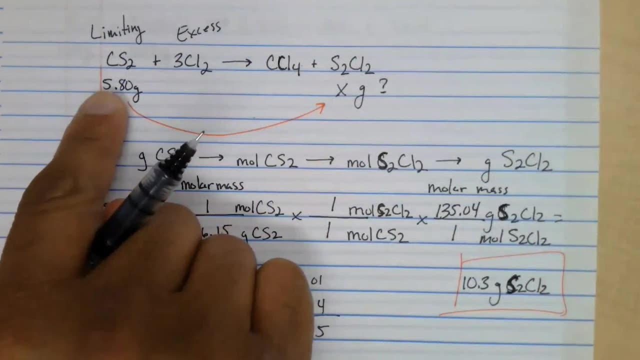 find the product. this is how much reactant we had find the product. this is how much. where am i right here? this is how. this is how much reactant we had find the product. this is how much reactant we had find the product. this is how much reactant we had. 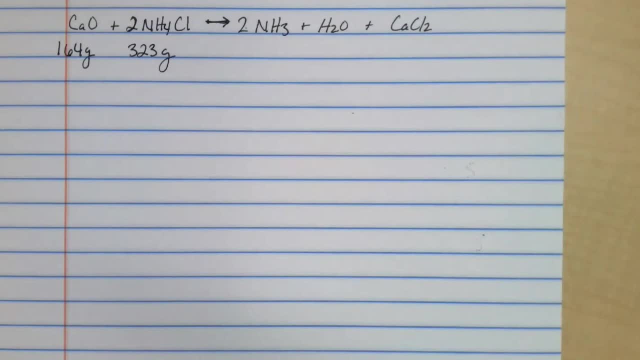 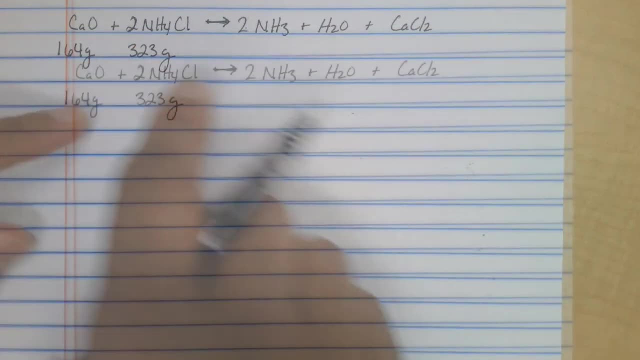 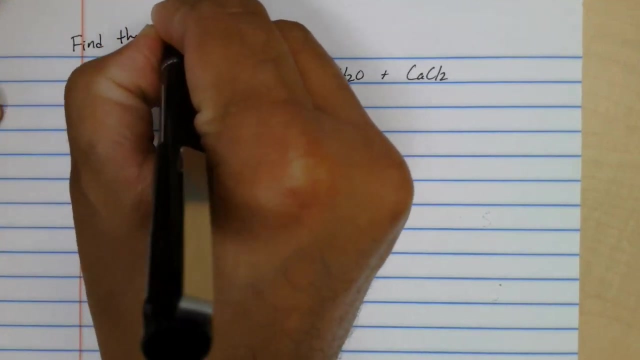 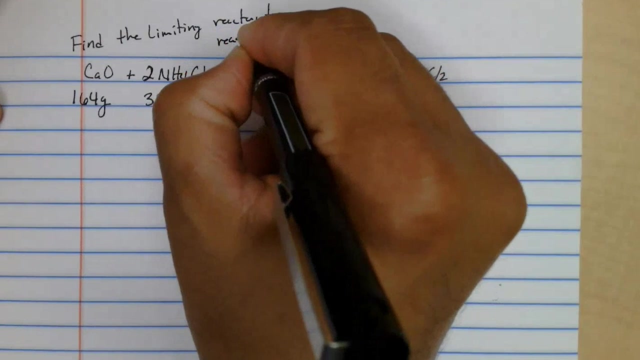 find the product. that's interesting here. they tell us: well, we have this much reactant of one reactant and then we have this much of the other. when you get a question like this, you must find the limiting reactant. sometimes it's called limiting reagent. it means the same thing: limiting reactant or limiting reagent. 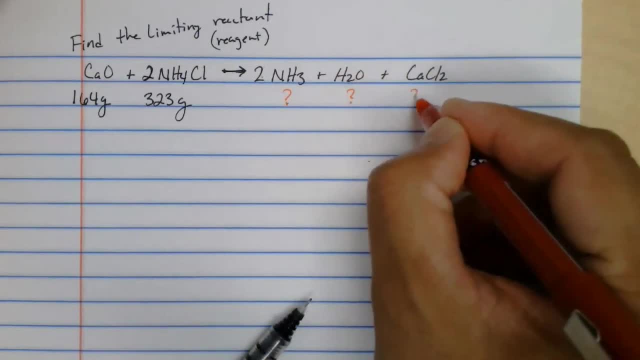 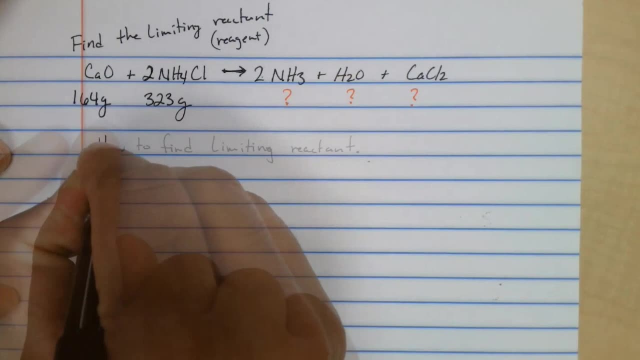 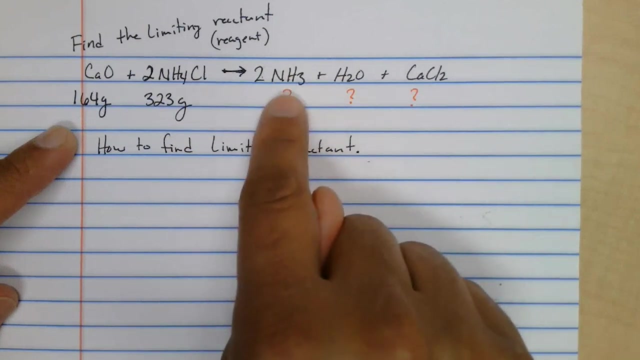 here and they want to know how much is produced. here's how you find the limiting reactant. pick one product, just pick one. i'll pick ammonia for this example. i'm just going to pick one and we're going to do a test: convert the calcium oxide. 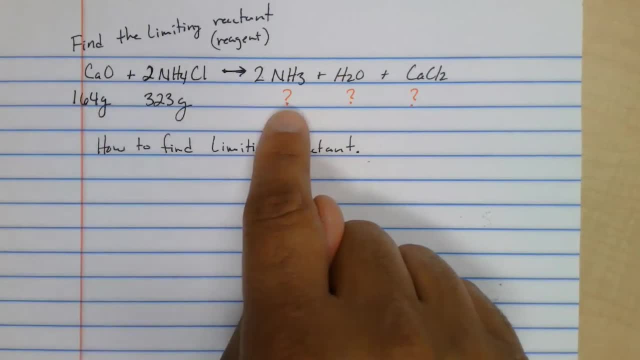 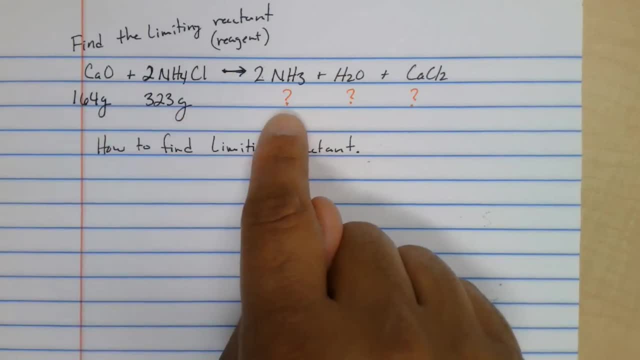 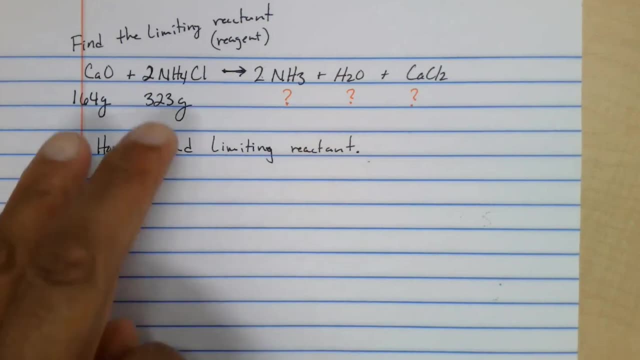 convert the ammonium chloride to ammonia and I'm going to get an answer: How many moles are produced. Let's do that, and then we're going to compare the moles. Whichever one produces the fewest is going to be limiting. 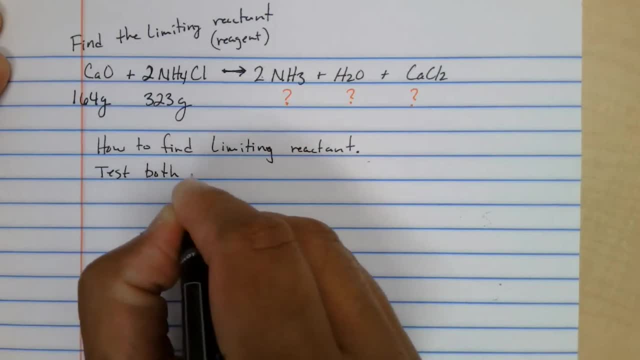 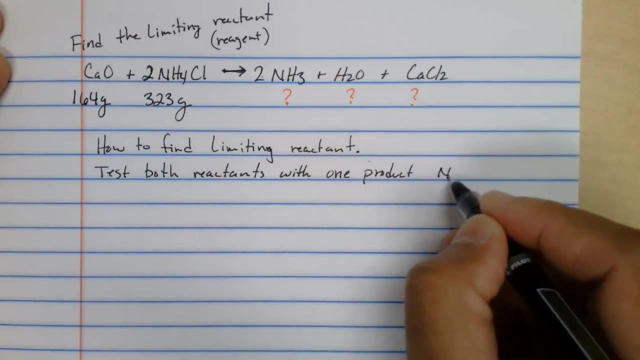 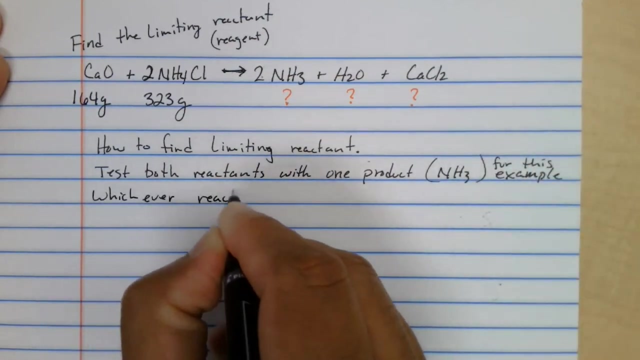 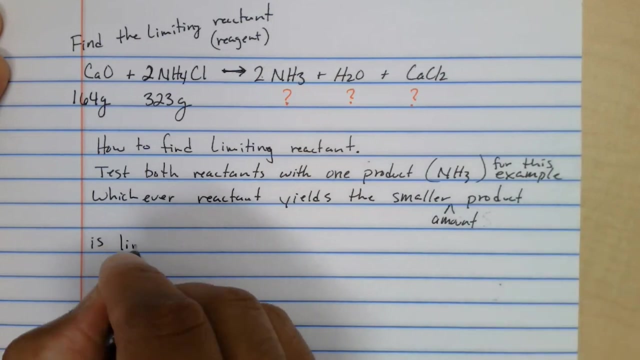 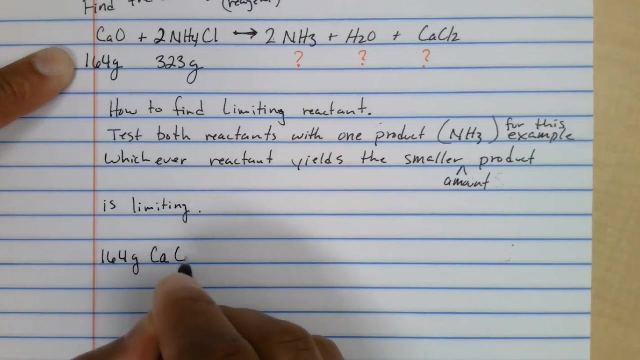 Test both reactants with one product. I'm going to pick ammonia for this example. Whichever reactant yields the smaller product is limiting. Let's start with 164 gram of calcium oxide In order to do this conversion, in order to use this ratio, I 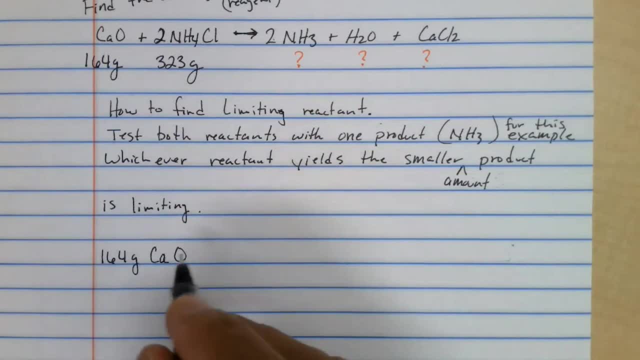 need to find the number of moles. So let's convert to the mole of calcium oxide. Let's cancel the gram of calcium oxide Using the molar mass. right here I can convert grams to moles. So we're good here. 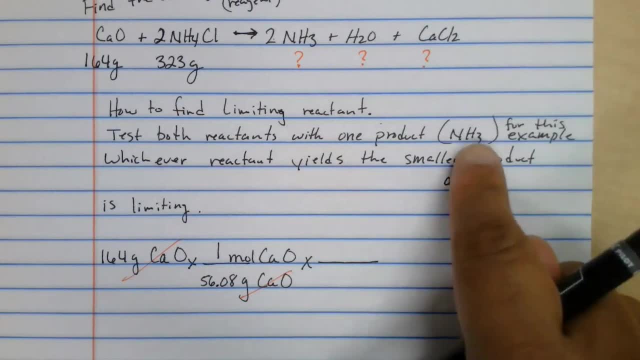 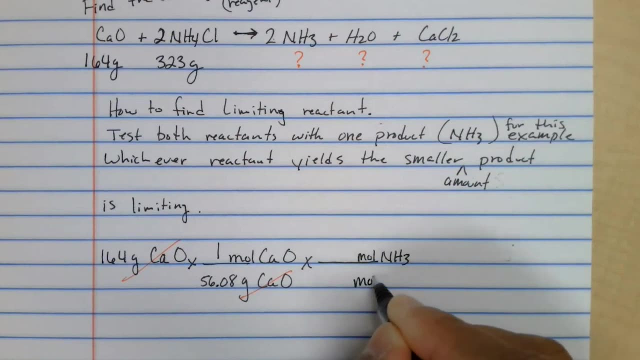 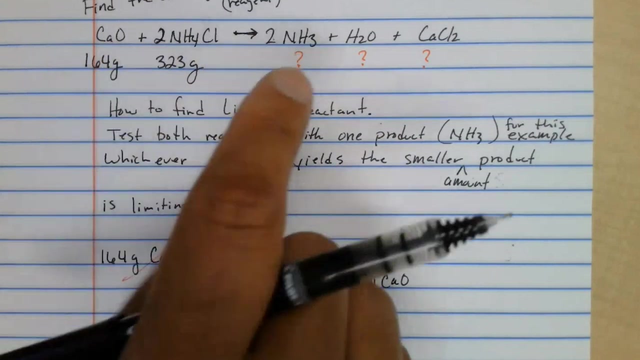 Now let's convert to one of the products. I'm going to pick ammonia for this example. So notice how I convert to mole of ammonia. Notice how I cancel the mole of the calcium oxide In this equation. that's already balanced, by the way. So be careful, Make sure the equations are balanced. 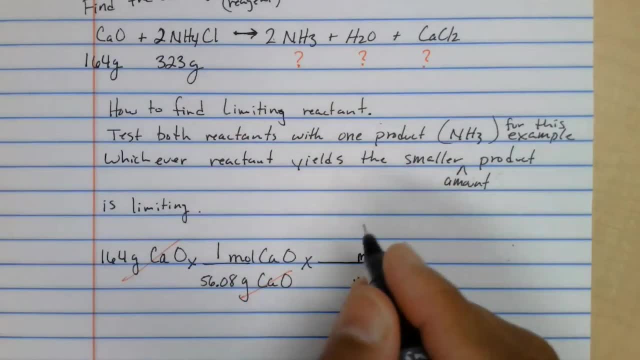 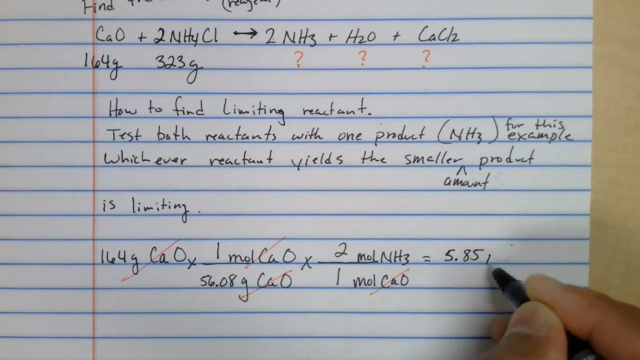 They're not always going to be balanced. In this case they balance them. for us, The ratio here is just two to one. right there, two to one. I start with three sig figs. So my answer here: 5.85 mole of NH3 can be produced from 164.. 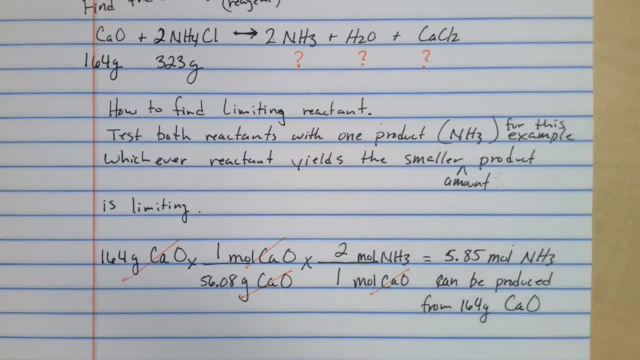 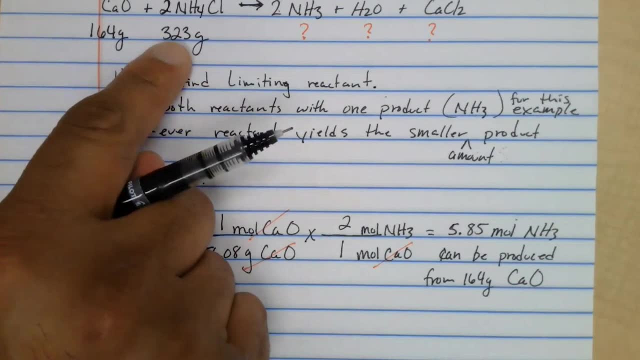 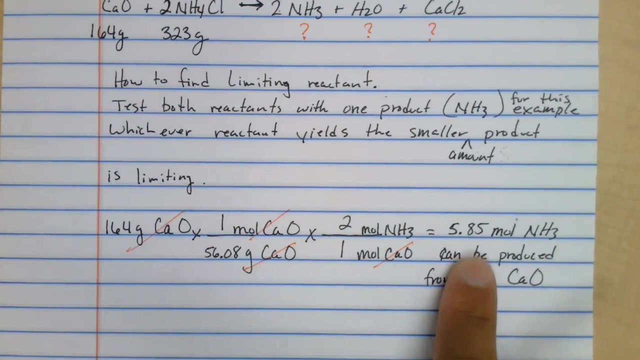 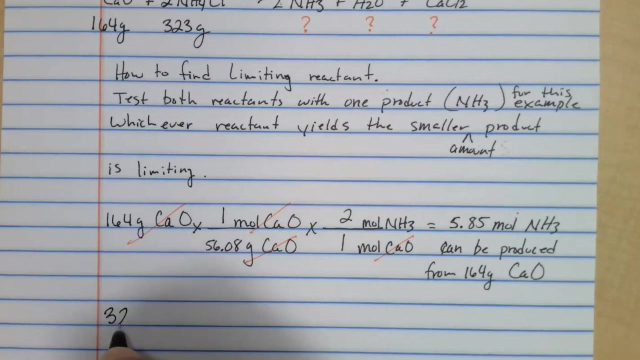 grams of the calcium oxide. We're not done yet. We still have to test the other one. I don't know which one is limiting. I have to do another test, But this is what I know so far. Let's do the next one: 3.23 grams of the ammonium chloride. 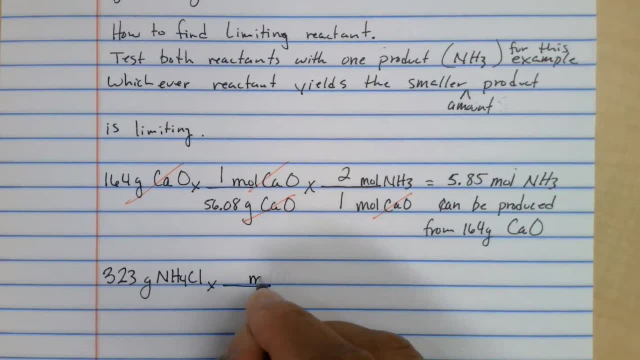 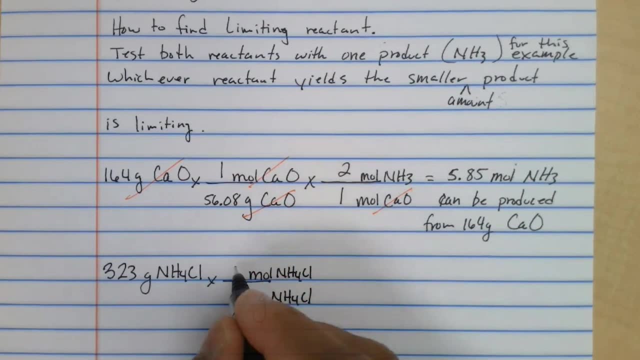 Let's convert to the mole of ammonium chloride and cancel the gram of ammonium chloride, The molar mass. here this comes out to 53.5 times. Now this one's a little bit different. The mole to mole ratio: here I'm going to do another test. 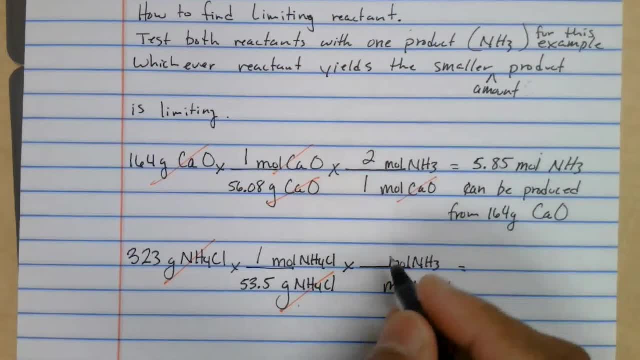 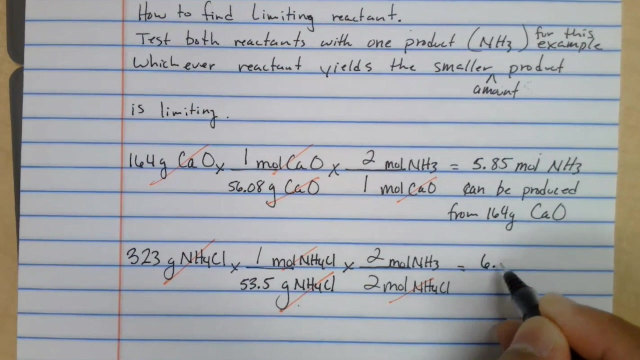 here is 2 to 2.. So for every 2 moles of ammonium chloride that reacts, you will always produce 2 moles of ammonia. So notice how this cancels here. So the answer here: 6.04 mole of ammonia. can be produced from 323 grams of ammonium chloride. Let's draw some conclusions. If I only had 164 grams of calcium oxide, I can produce 5.85 moles of ammonia If I have 323 grams of ammonium chloride. 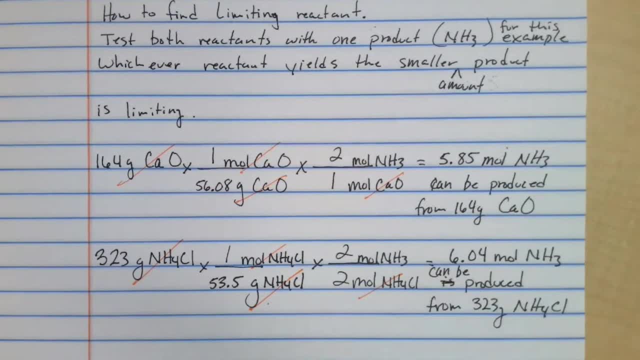 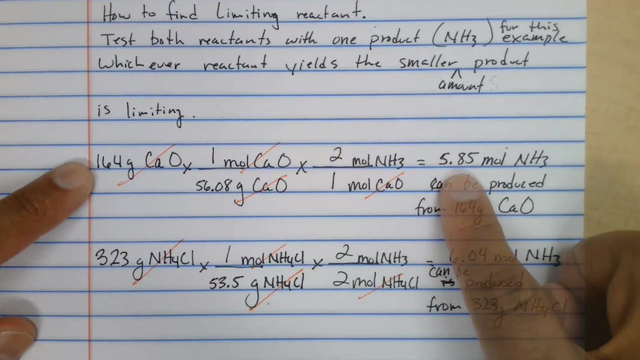 I can produce 6.04 moles of ammonia. So you can imagine if these two things react as soon as you get to the smaller number, then the 164 grams of calcium oxide has now run out. The calcium oxide that produces the fewest amount is the limiting reactant. Now notice here: 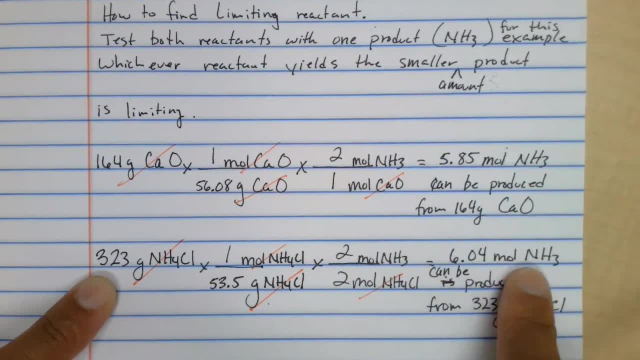 the ammonium chloride can give you more than the 2 moles of ammonia. So if I only had 6.04 moles of ammonia, the calcium oxide can give me some more ammonia. But we never get to this number here, because as soon as we get to the 5.85, then the calcium oxide has run out. 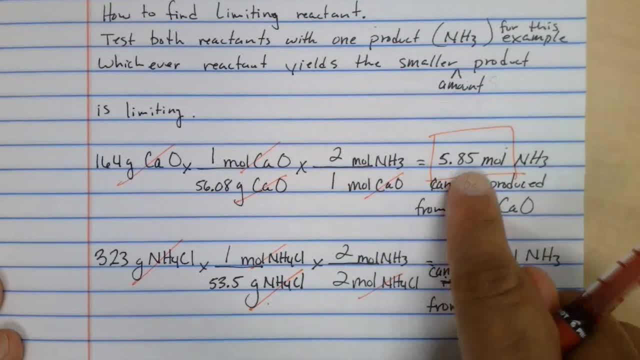 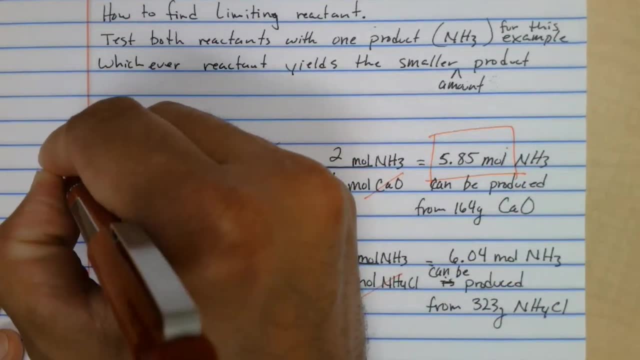 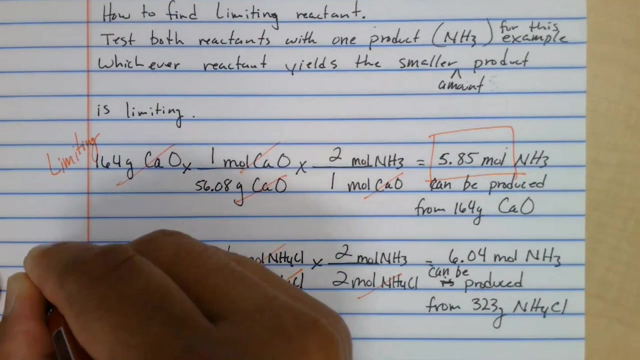 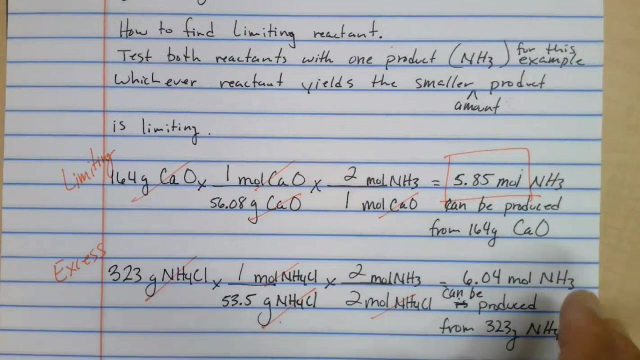 So let's draw some conclusions here. 5.85 mole is how much we can get. Calcium oxide is limiting, Calcium oxide is limiting And the ammonium chloride is the excess. Now that we know that calcium oxide is the limiting reactant, we use the limiting reactant. 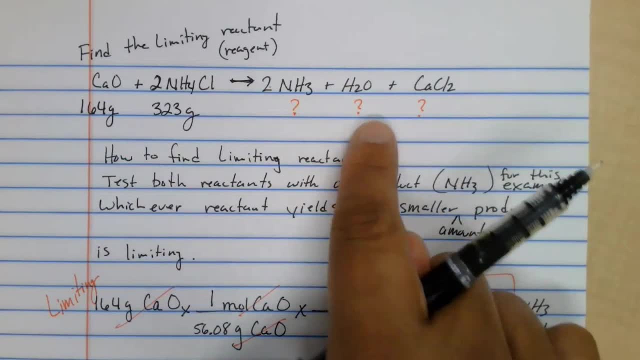 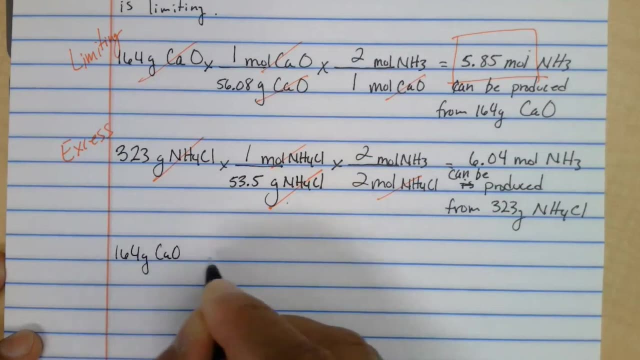 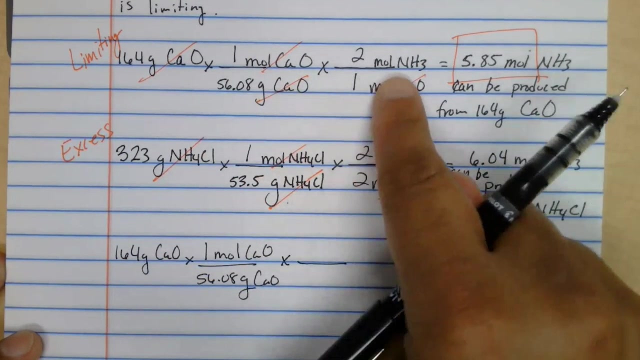 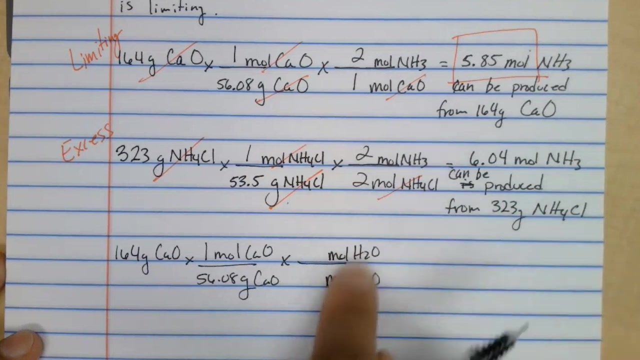 to find everything else. So when they ask us how much water? so watch this. 164 convert to moles. So I'm just copying what I have right here. but now look at this. I'm going to convert to the mole of water and cancel mole of the calcium oxide. So notice here. 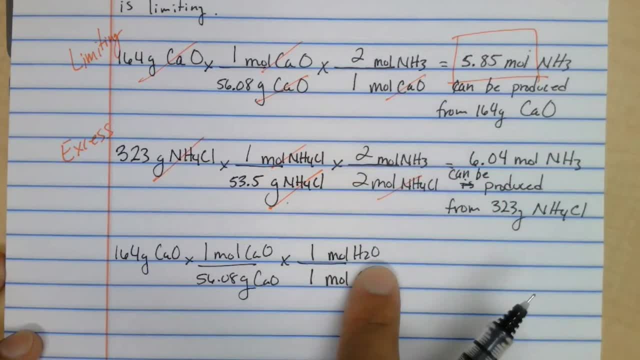 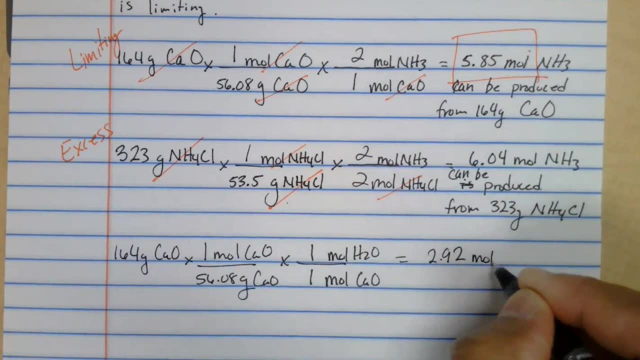 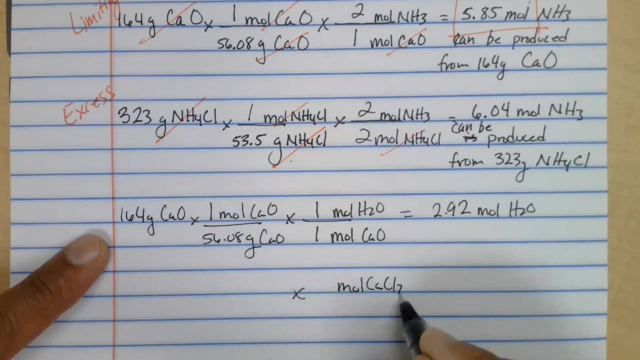 I've changed what I'm looking for, So I'm going to convert to the mole of water and cancel mole of the calcium oxide. So three sig figs, 2.92 mole of water, We can convert to mole of the calcium chloride And if 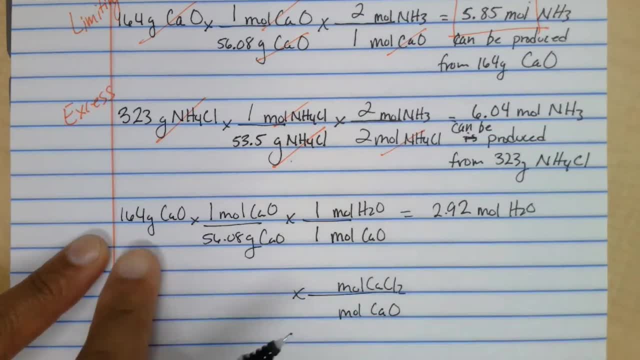 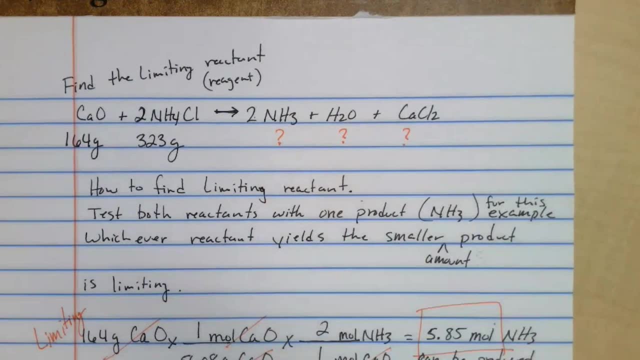 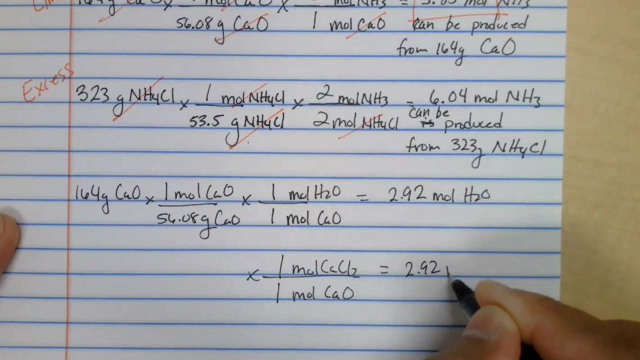 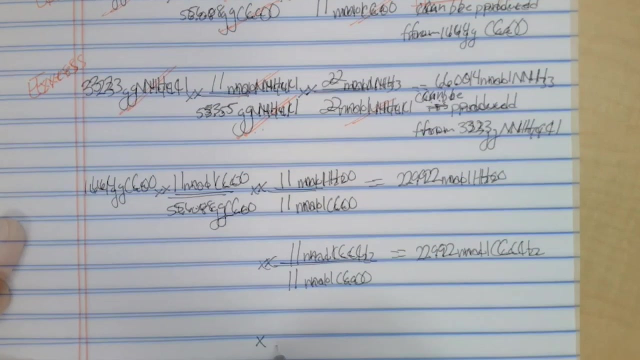 you look closely? right, instead of going to water we can go to calcium chloride. But if you look closely, what do you notice? It's the same ratio, right? So there you go, It's actually the same answer. Notice how nothing changes there, Just this last part. right here I'm going to do the same thing.